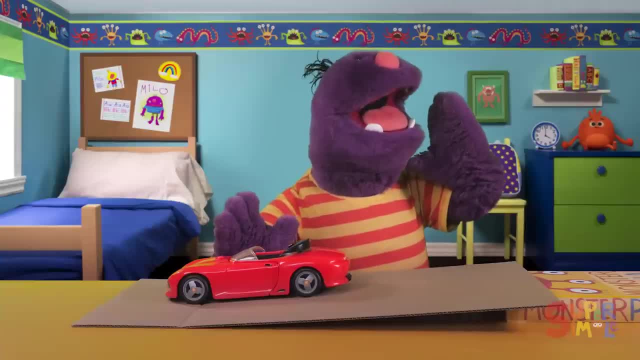 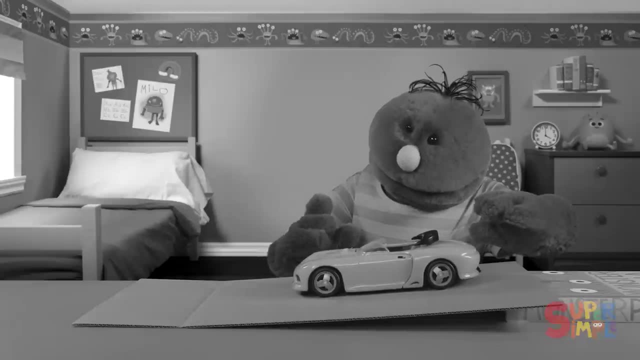 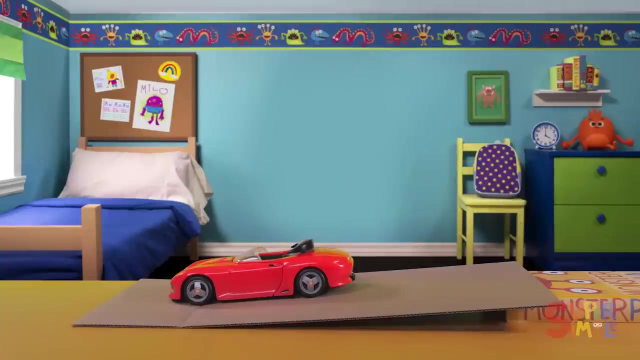 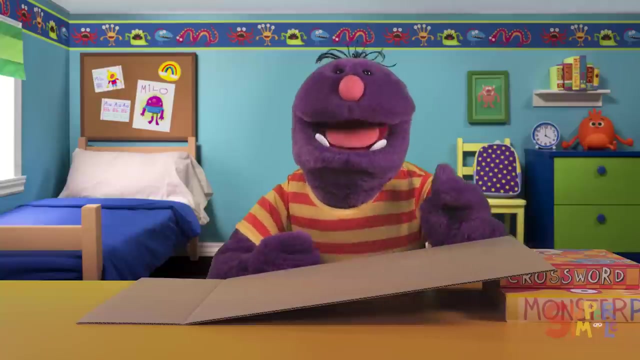 Let's watch it again. Instant replay. Maybe I need more books. Look how high the ramp is. I'm gonna race the car again And what do you think will happen? Will the car go faster, Slower Or the same speed as it did before? 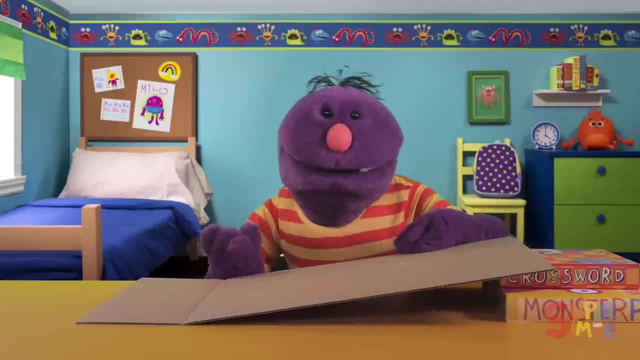 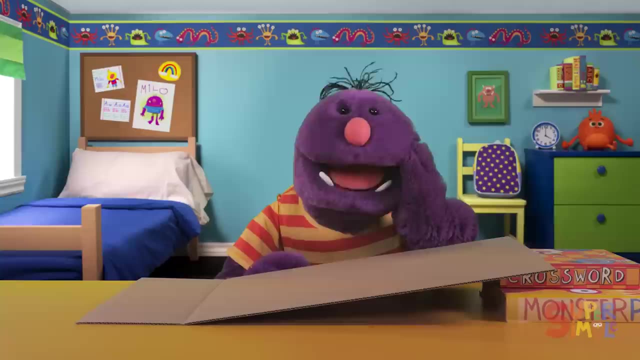 I know the answer because we did it in monster school. But you take a guess. Let's see what happens. On your mark: get set. go On your mark, get set. go On your mark, get set go. 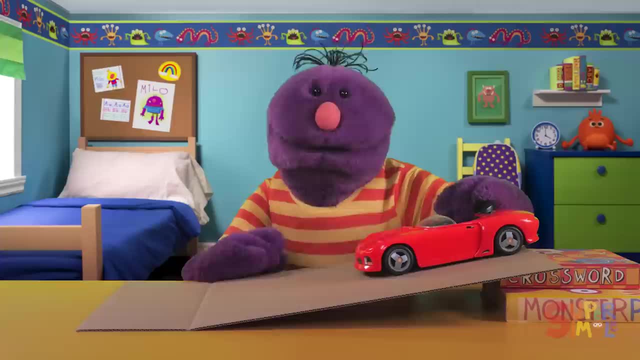 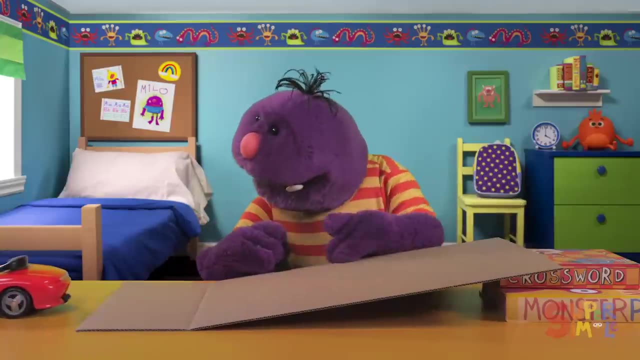 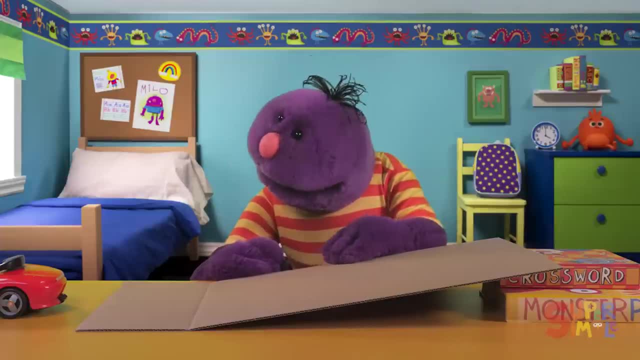 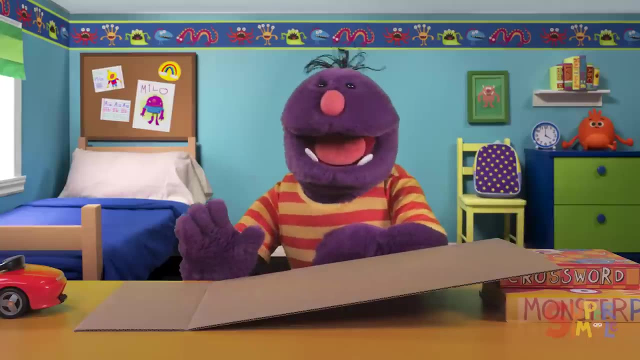 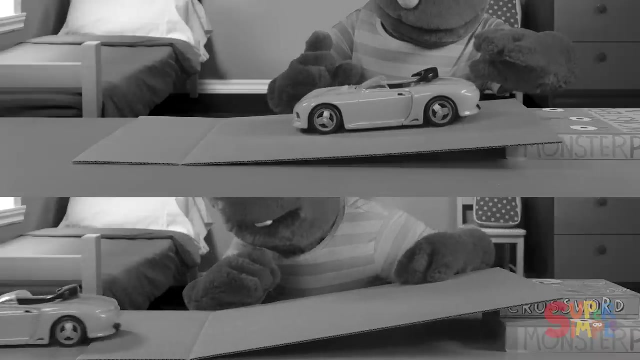 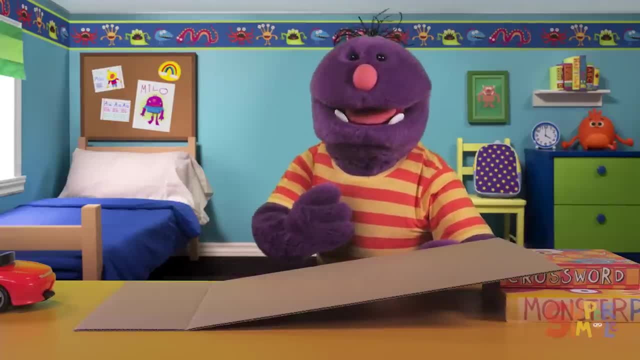 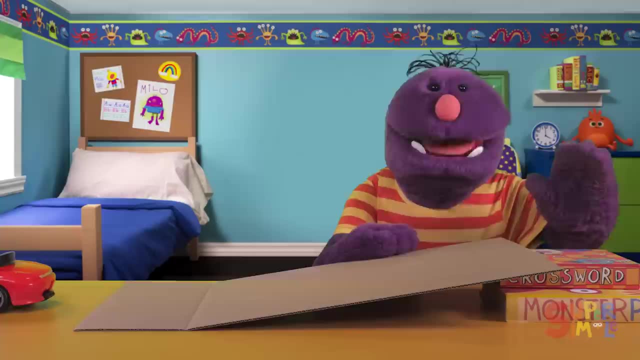 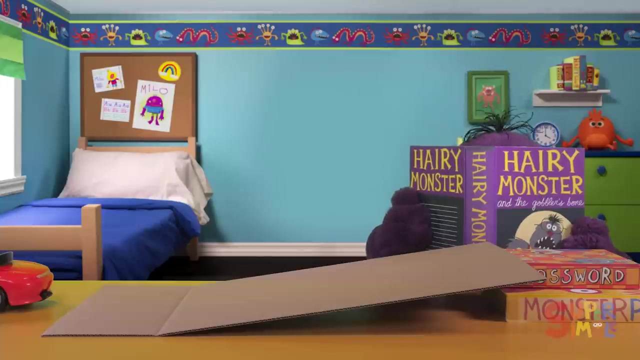 When I moved the ramp higher, the car went faster. Zoom, Zoom. Let's add a third book and see what happens. Great Look, Riveting. A real page turner. A real page turner. I almost don't want to use it to. 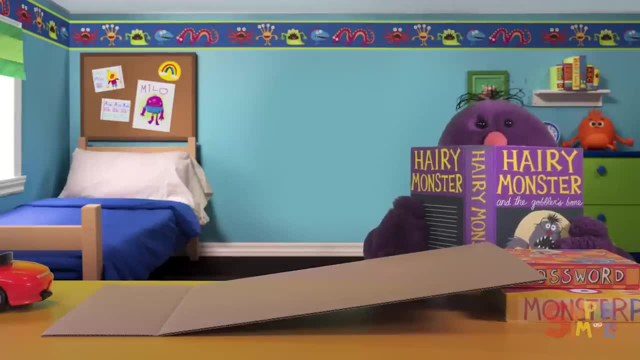 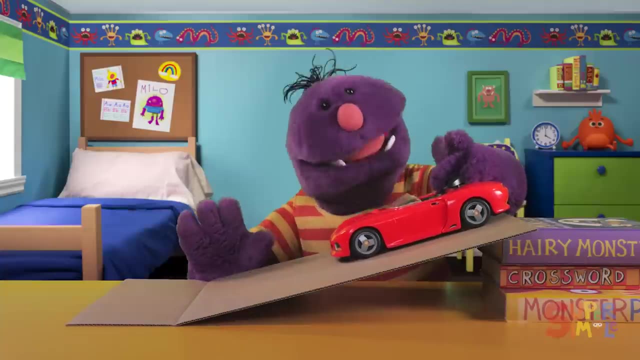 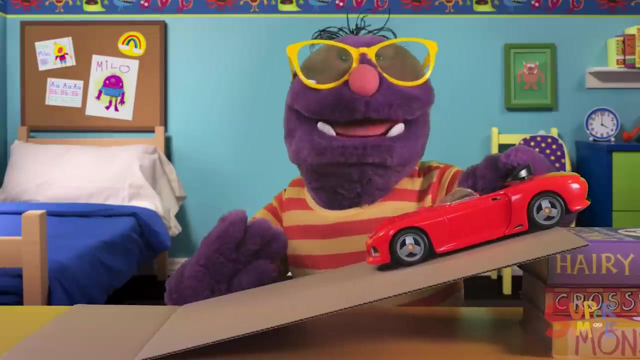 raise the ramp Almost. Look how high it is. Look how high it is. It's so treacherous. It's race time. Will this car go the fastest yet? Will this car go the fastest yet? I have the need for speed. 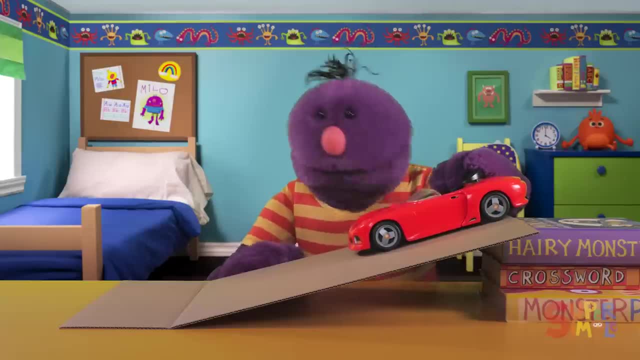 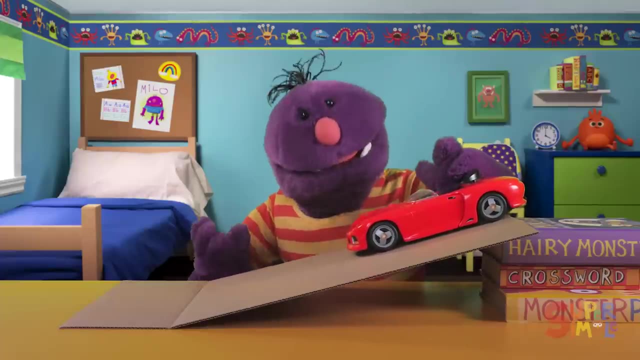 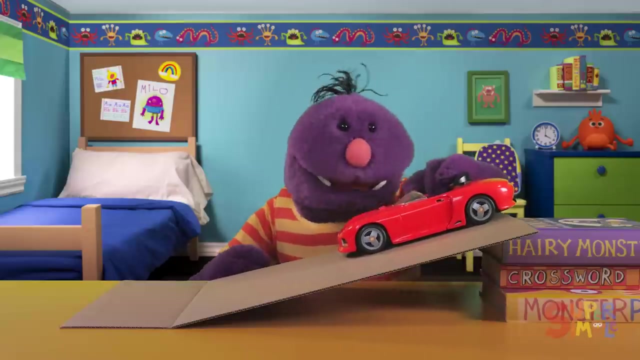 I have the need for speed. Countdown with me. Ten, Nine, Eight, Five, Two, Wait, wait, wait. That's wrong. Let me try that again. Ten, Thirteen, Niner, No, no, no, no.